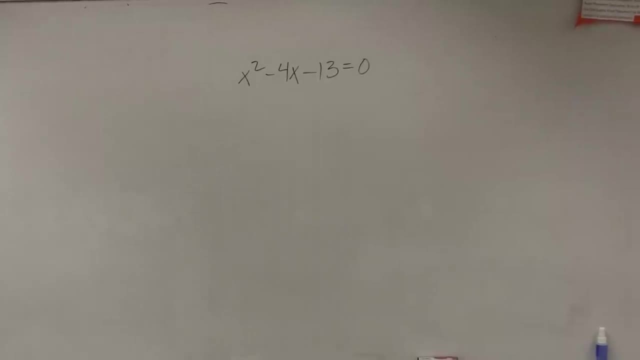 What we're going to do for this problem is we're going to do exactly kind of what we did before, in two different steps, All right. so we're going to do the same exact stuff, but we're going to kind of break it up. So what we have is: I have x squared minus 4x minus 13 equals 0.. Now remember: 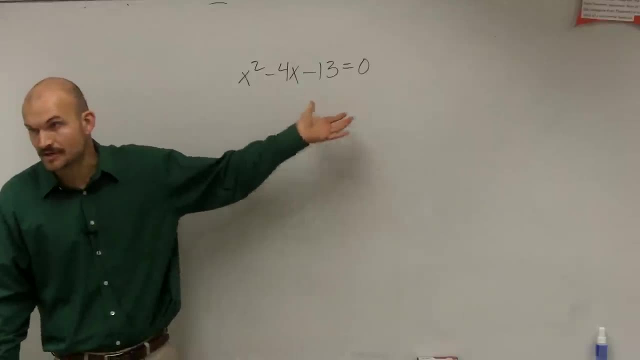 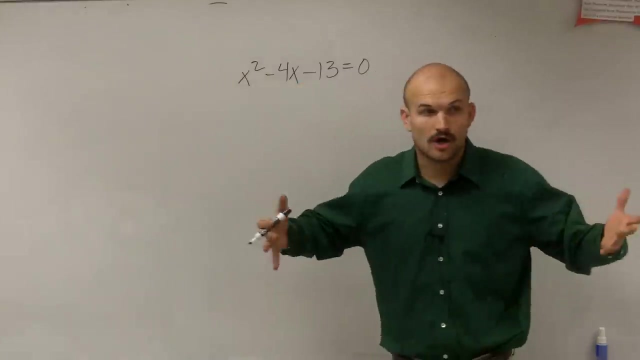 you always want to see. you know, can you factor this? And unfortunately this cannot be factored in our normal case that we've worked on And it's said to solve by completing the square. Now, remember, completing the square involves creating a perfect square trinomial, So you have to create 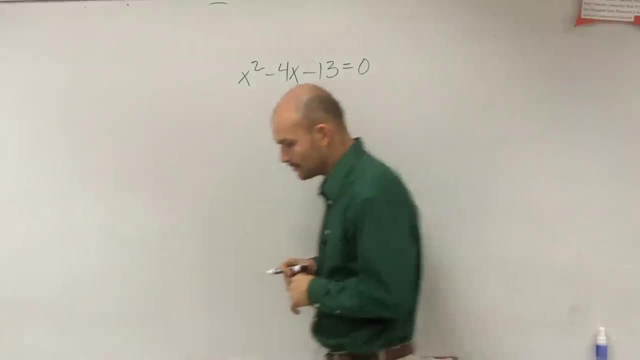 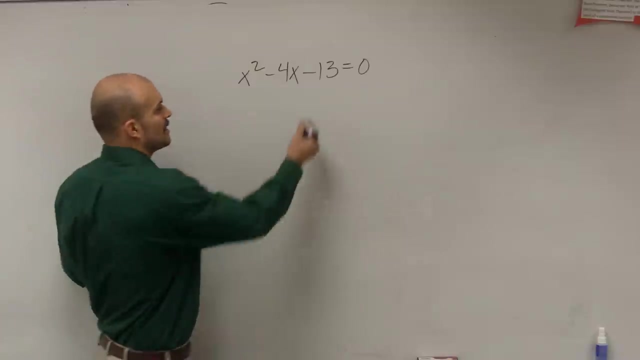 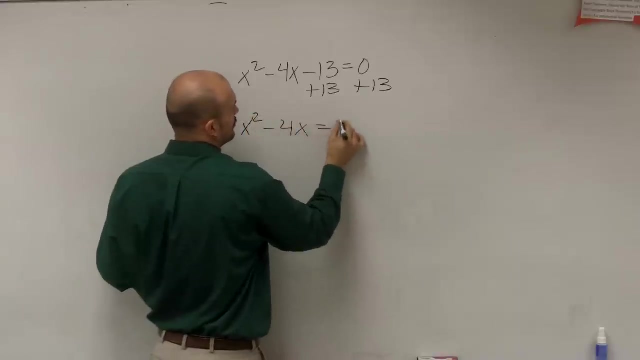 a perfect square trinomial. So to do that, what we're going to do is- we got to make sure we will- we got to create a perfect square trinomial. So the first thing I'm going to want to do is get my constant to the other side. So I have x squared minus 4x equals 13.. 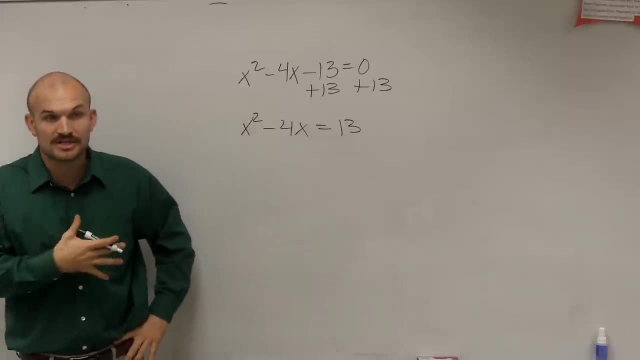 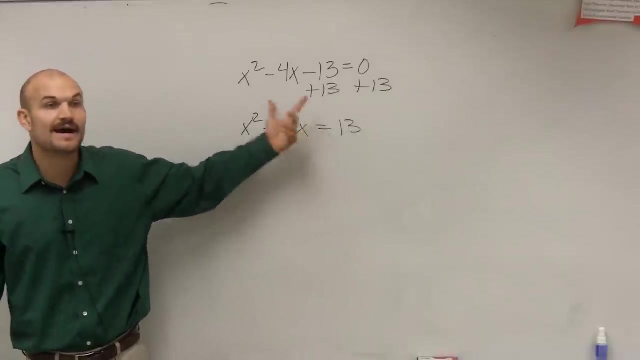 All right. so now, what we're going to do is exactly like what we just did: we are going to find the value c. that will create a perfect square trinomial. So we got to find the value. We got to find a new value. So, to find our new value, what we're going to do is exactly what. 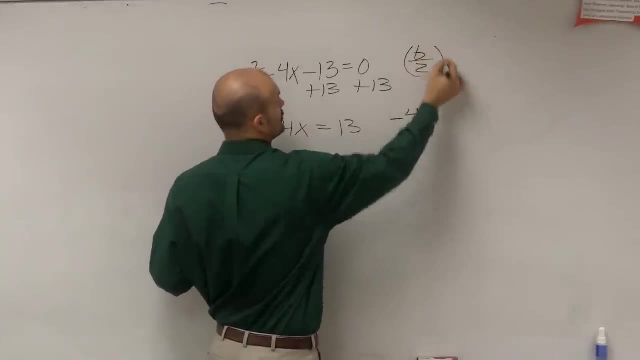 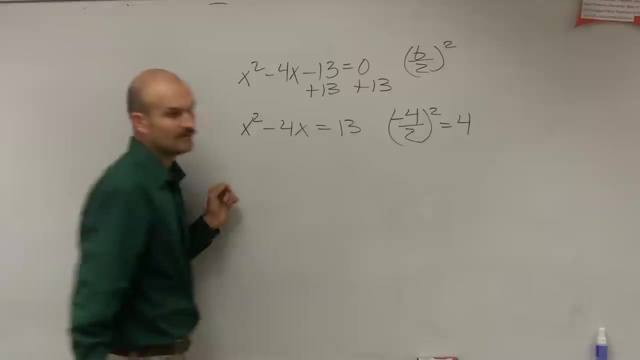 we did before. Take our b divided by 2 and square it. So we take negative 4 divided by 2 and square it, And we'll get positive 4, correct? So therefore we write x squared minus 4x plus 4.. 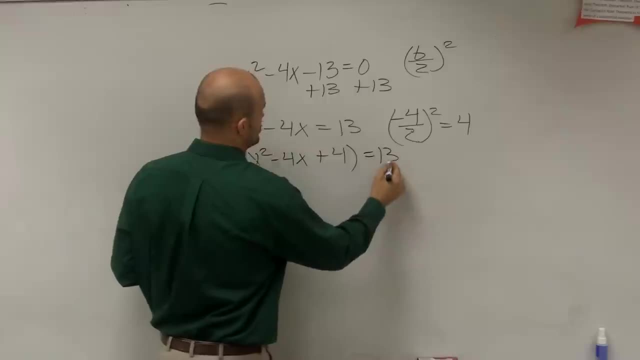 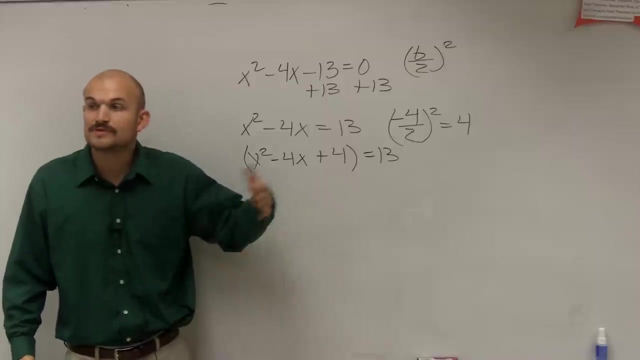 Sorry, Equals 13.. Okay, Now going back to solving equations. All right, if you do something to one side, what do you always have to do on the other side? Exact same thing. So what did we do over here? We added 4.. So what do you think you're going to want to do on the other side? Add 4.. 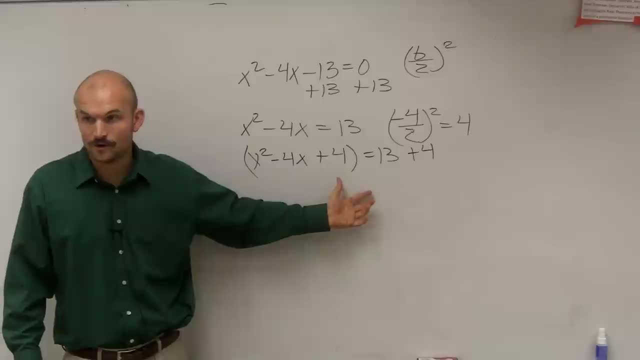 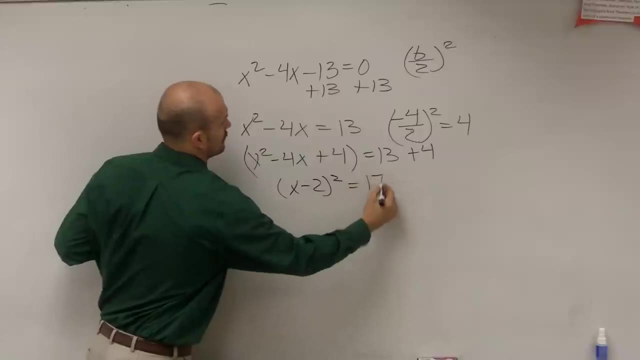 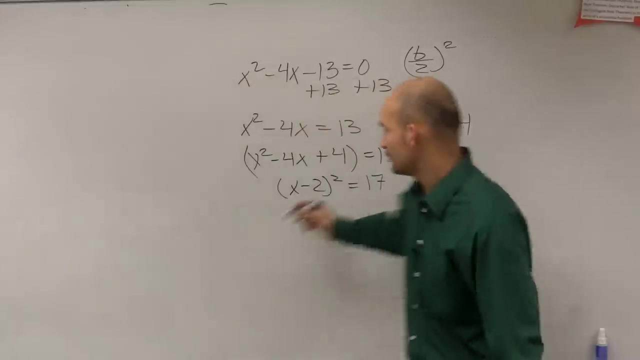 Okay, Now, since we've created a perfect square trinomial, we can write a perfect square trinomial And we can write a perfect square trinomial, So we're going to write this as a perfect square. Does everybody follow me? Remember to always find the perfect. 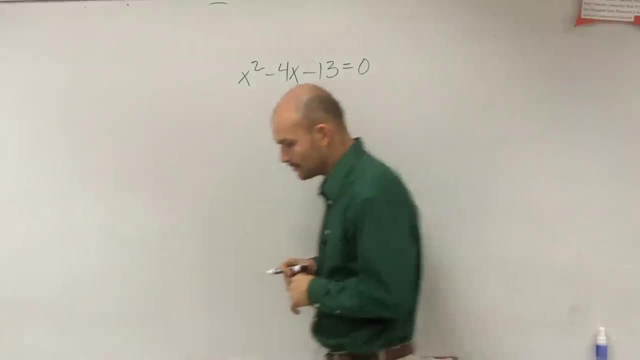 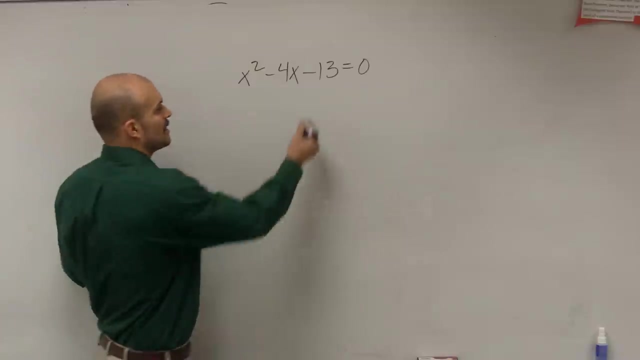 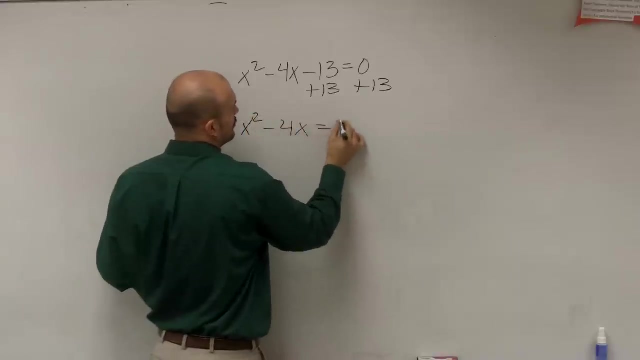 a perfect square trinomial. So to do that, what we're going to do is- we got to make sure we will- we got to create a perfect square trinomial. So the first thing I'm going to want to do is get my constant to the other side. So I have x squared minus 4x equals 13.. 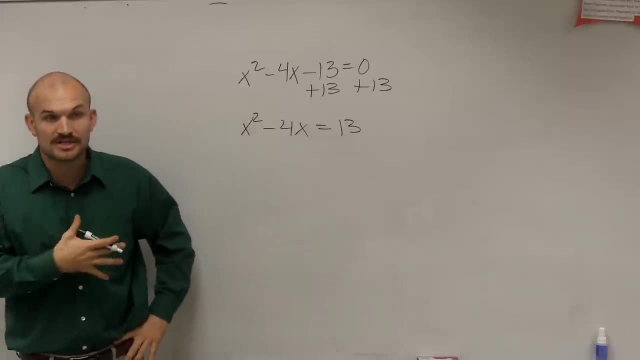 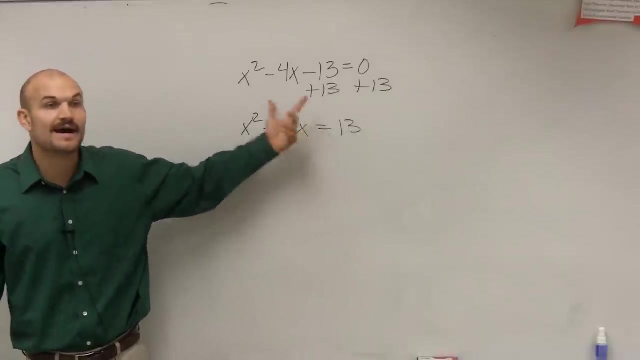 All right. so now, what we're going to do is exactly like what we just did: we are going to find the value c. that will create a perfect square trinomial. So we got to find the value. We got to find a new value. So, to find our new value, what we're going to do is exactly what. 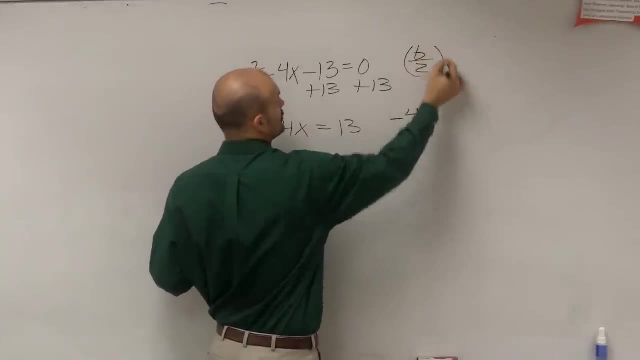 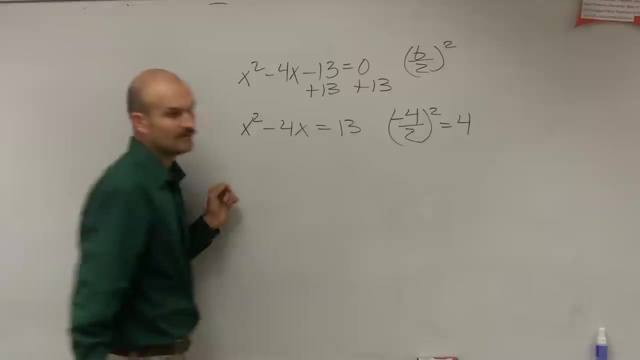 we did before. Take our b divided by 2 and square it. So we take negative 4 divided by 2 and square it, And we'll get positive 4, correct? So therefore we write x squared minus 4x plus 4.. 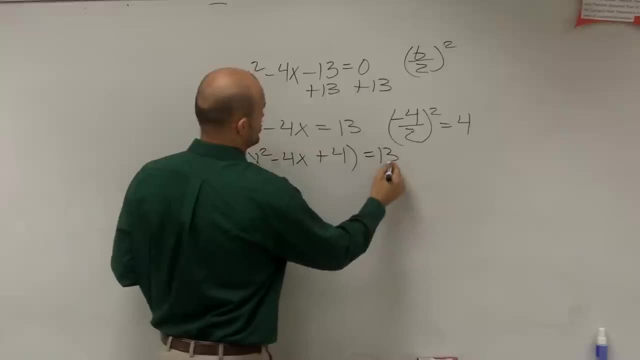 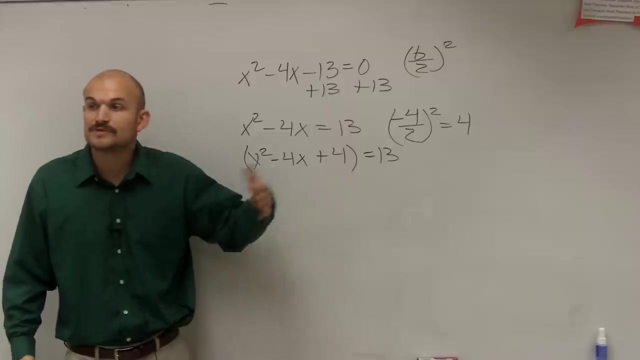 Sorry, equals 13.. Okay, now going back to solving equations. All right, if you do something to one side, what do you always have to do on the other side? Exact same thing. So what did we do over here? 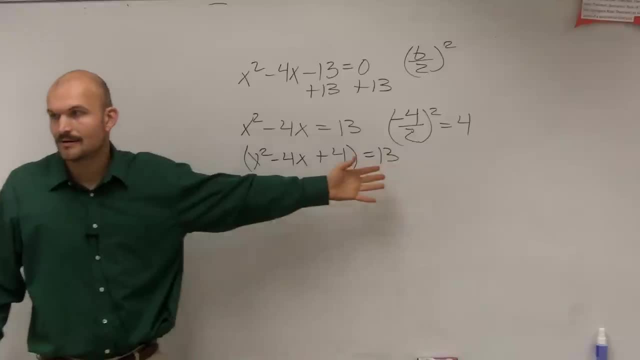 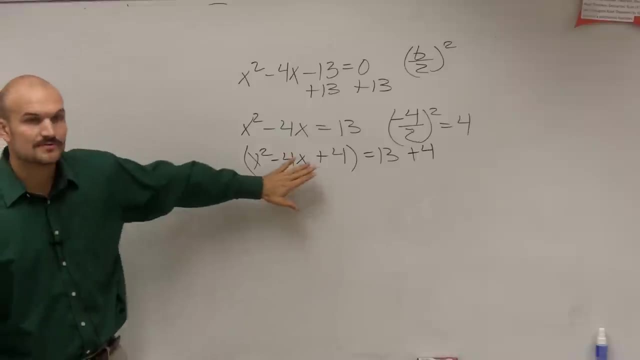 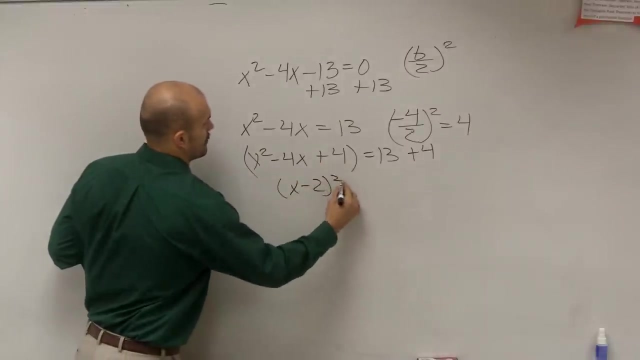 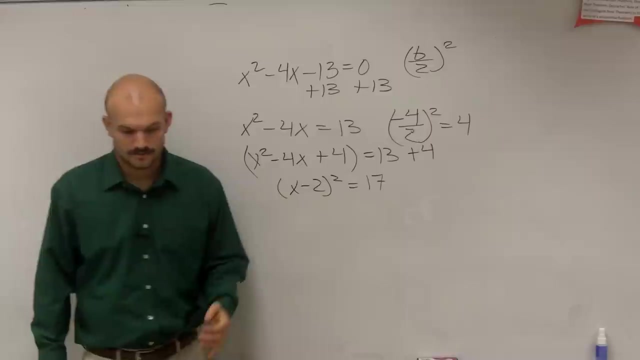 We added 4.. So what do you think you're going to want to do on the other side? Add 4.. Okay, now, since we've created a perfect square trinomial, write this as a perfect square. Does everybody follow me? Remember to always find the perfect. 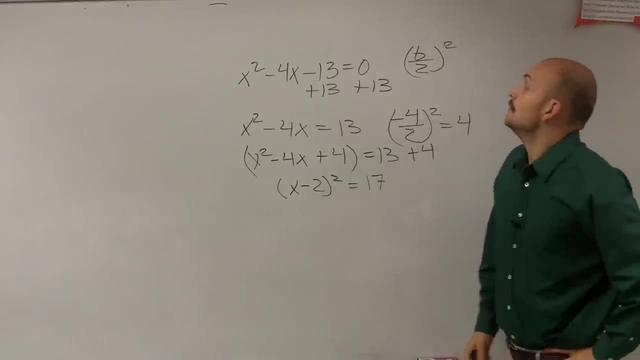 square. just take your b and divide it by 2.. Does everybody follow me so far with this? Remember with 13, I moved to the other side And then remember since I added 4 on the left side to create a perfect square. 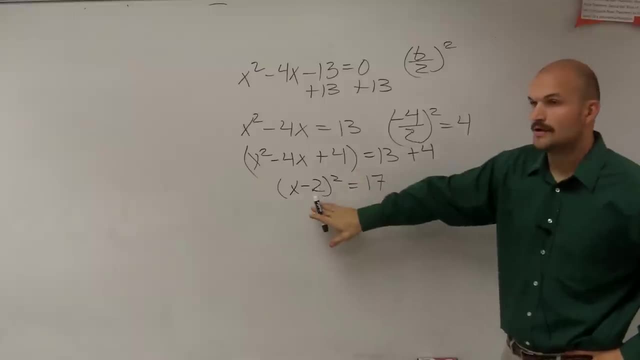 I had to make sure I added 4 on the other side. Now, how many x's do we have, Ricardo? How many x's do I have in this equation 1. Can we solve with just 1x By using inverse operations? Yeah, 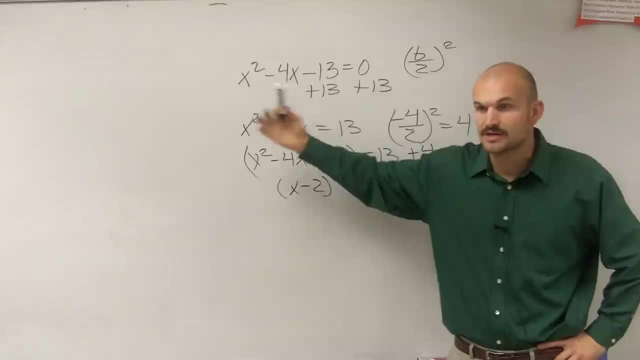 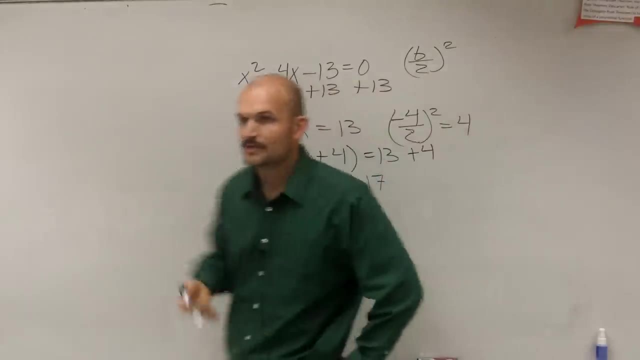 You can't solve for x when you have 2x's right. You either combine like terms, which you can't do, or you have to factor. But now I only have 1x. I can use my inverse operations. So the first inverse 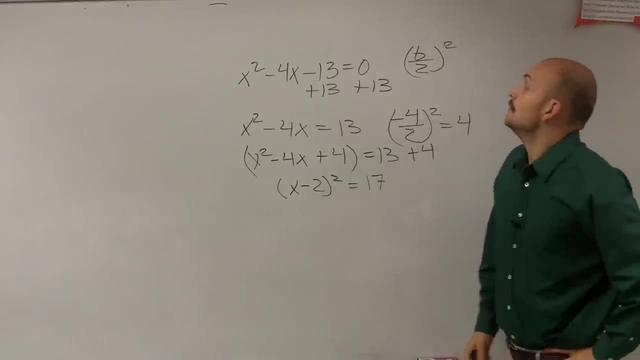 square. just take your b and divide it by 2.. Does everybody follow me so far with this? Remember with 13, I moved to the other side And then remember since I added 4 on the left side to create a perfect square. 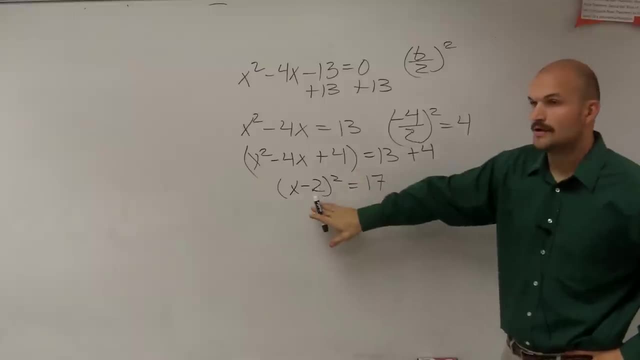 I had to make sure I added 4 on the other side. Now, how many x's do we have, Ricardo? How many x's do I have in this equation 1. Can we solve with just 1x By using inverse operations? Yeah, 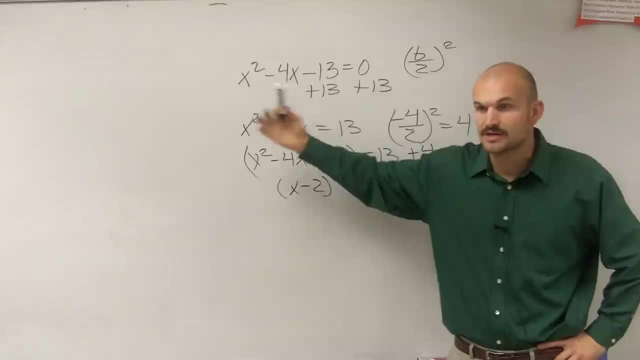 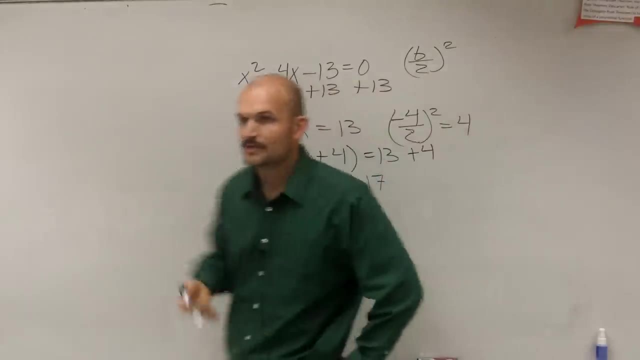 You can't solve for x when you have 2x's right. You either combine like terms, which you can't do, or you have to factor. But now I only have 1x. I can use my inverse operations. So the first inverse 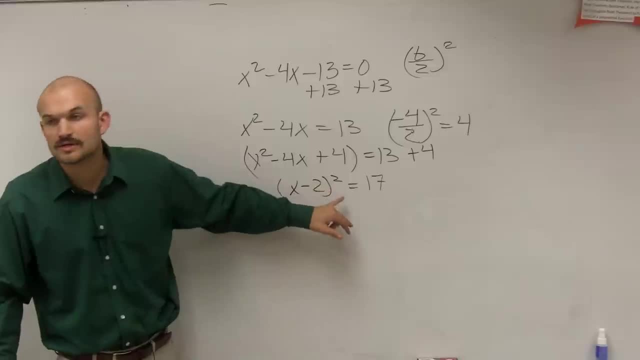 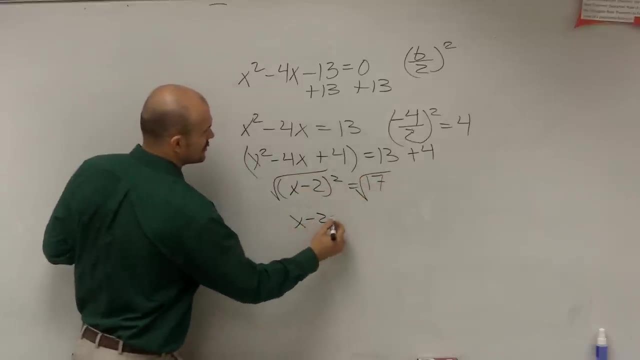 operation I have to do is my: I have to undo. I have to undo this exponent of 2.. So I have to take the square root on both sides. Therefore, I have x minus 2 equals plus or minus the square root of 17.. Now, the square root of 17. 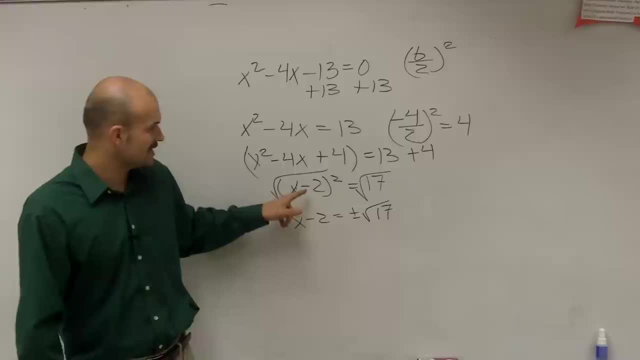 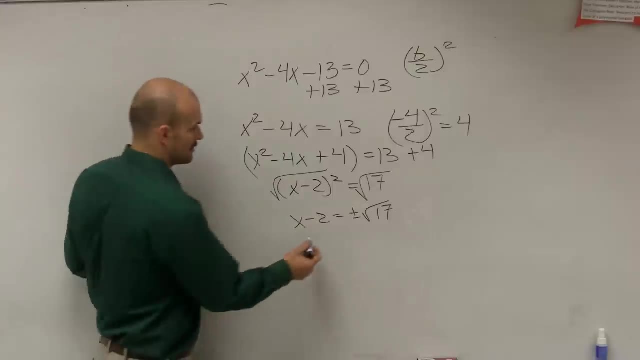 cannot be simplified, so we're going to leave it like that. Just remember, since I introduced the square root, I have to take the plus or minus of the number. Now to get x by itself, I'm just going to add 2.. 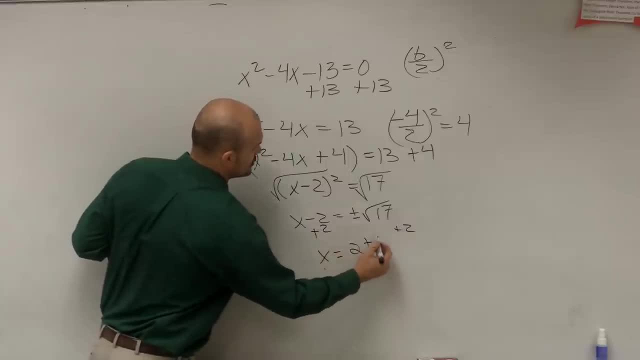 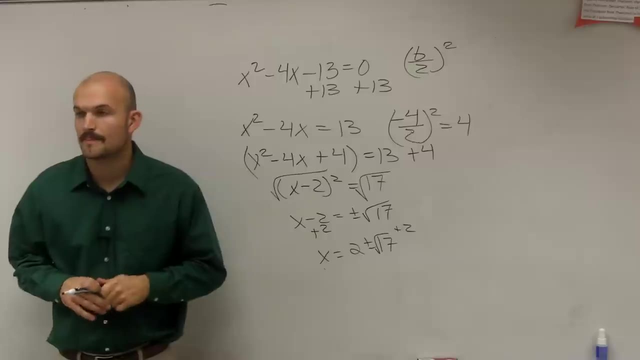 So therefore, my final answer is: x equals 2 plus or minus the square root of 17.. Yes, Or it can be simplified Like the square root of 8.. You know, you could simplify that as like 2 square root of 2.. Right, Just leave it like that. 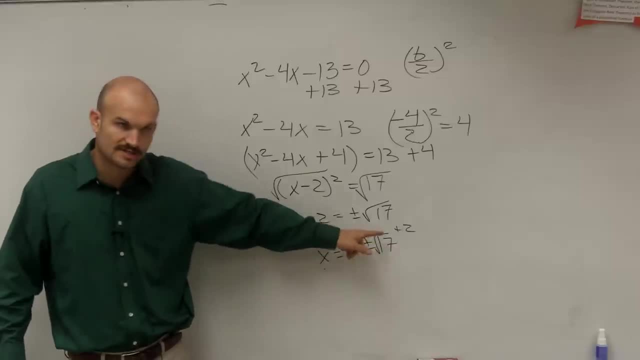 Yep, And that will be your final answer. And notice you're going to have two answers: 2 plus square root of 17 and 2 minus the square root of 17.. But we're not doing decimals. Just leave it like that. Yes, 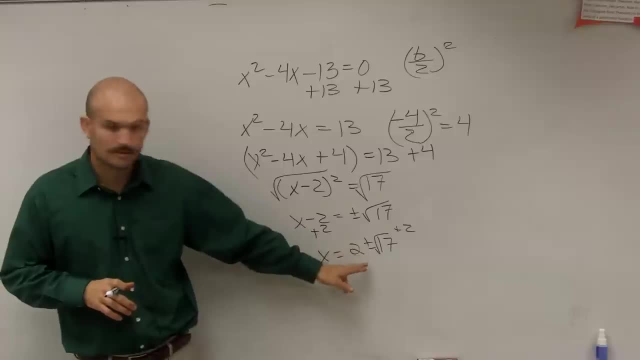 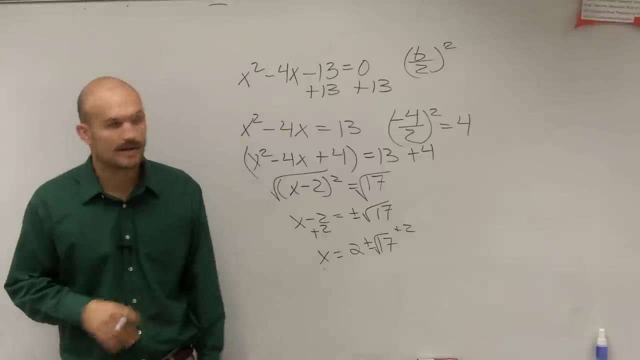 Would it be wrong if you left it like what Here? No, that's how I want you to leave it, Just like that. I don't want you doing decimals. I want the exact value. Okay, And that's it. Yes.